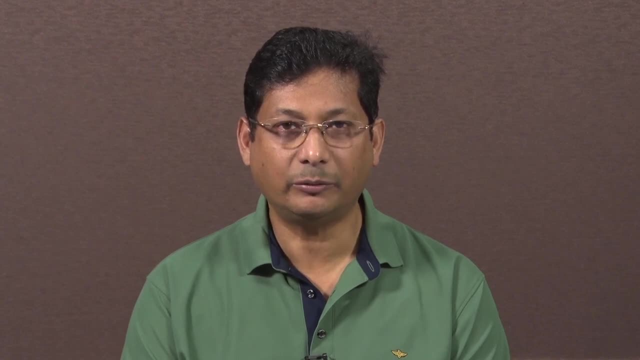 important concept, that is, the Gaussian mixture model and the expectation maximization algorithm. In most of the engineering and other applications, like in signal processing, communication, machine learning and many other applications, we consider a Gaussian distribution for representing a data distribution. That means a particular data distribution can be approximated by a. 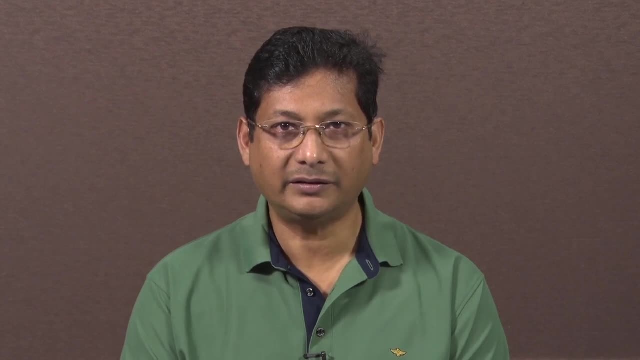 Gaussian distribution. It has many advantages. So one advantage is that Gaussian distribution is very closer to the natural distribution. That is the first advantage. Another important point is the mathematical manipulations, for Gaussian function is easy. So if I want to determine the derivative of a Gaussian function, 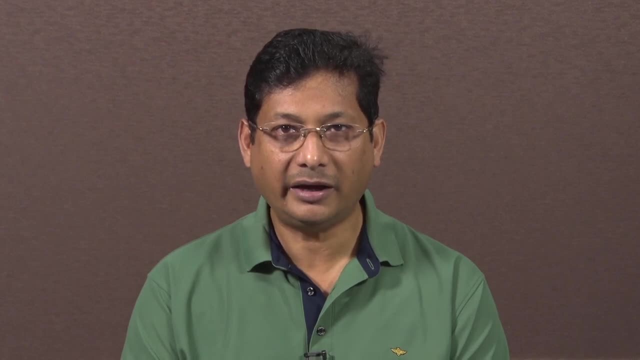 it is easy to determine this derivative. I can determine the nth order derivative of a Gaussian function Like this. there are many advantages of considering a Gaussian function In case of a complex data set, or maybe the distribution. it is not possible to represent this data set by a single Gaussian, So for this I have to consider multiple. 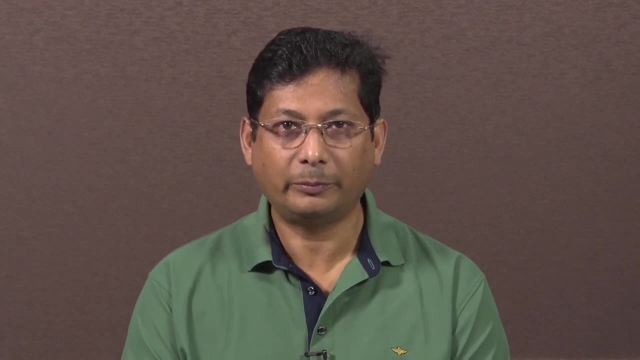 Gaussians, That means the mixture of Gaussians. So for a complex data distribution it is not possible to represent the distribution by a single Gaussian. We have to consider multiple Gaussians and that is the mixture of Gaussians. Now, in case of a Gaussian distribution, or in case of the Gaussian density, I have 2. 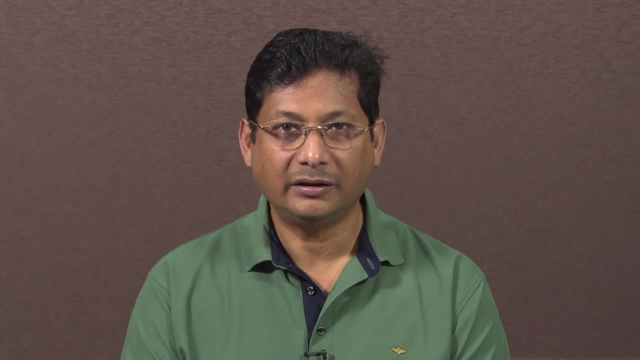 parameters mean. another one is the variance. If I consider the multidimensional case. one is the mean vector and another parameter is the covariance matrix. So these parameters I can determine by some estimation techniques, like maximum likelihood estimation technique I can apply to determine the or to estimate the values of the parameters: the mean vector and the. 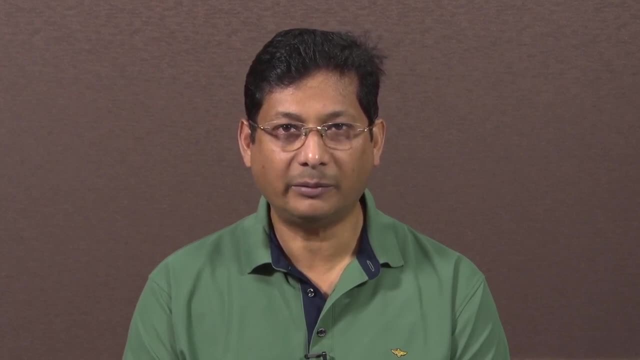 covariance matrix. In case of a Gaussian mixture model I cannot apply the maximum likelihood estimation technique because it cannot give a close form of solution. So for this I have to apply some iterative algorithm. and one algorithm is very popular algorithm is expectation maximization algorithm. So in this class I will be discussing first 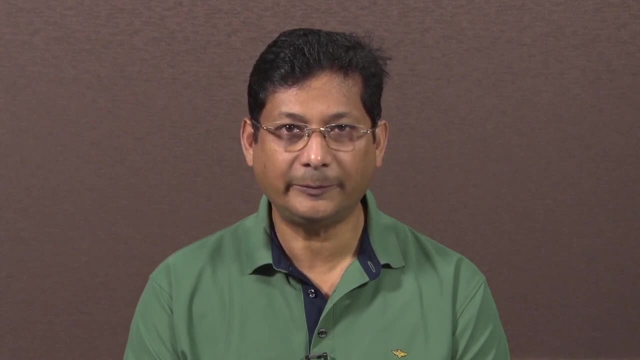 the concept of the Gaussian distribution, that is, the Gaussian density. and after this I will be discussing the concept of mixture model, that is, the Gaussian mixture model. and after this, To determine the values of the parameters, I will show one iterative algorithm, that is the expectation maximization algorithm. So let us begin this class. 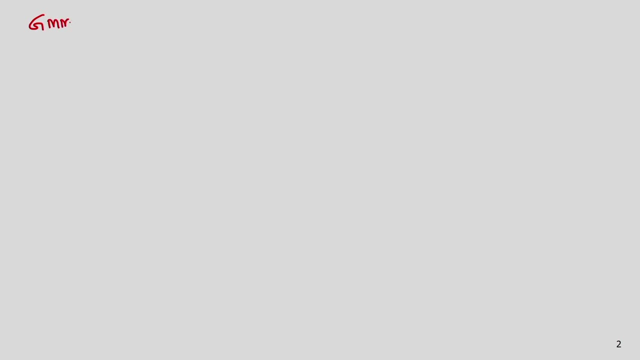 So ZMM, that is the Gaussian mixture model, using EM. EM means the expectation maximization technique. So first let us consider a Gaussian distribution. So it, it is the one dimensional distribution. So this density, the Gaussian density, I can write like this: It has two parameters: one: is the mean and another one is the variance. So it clear. So positive, So positive, Okay, So positive example. So negative is one, see your one. So you can also give a double相 in here for a common triad value. 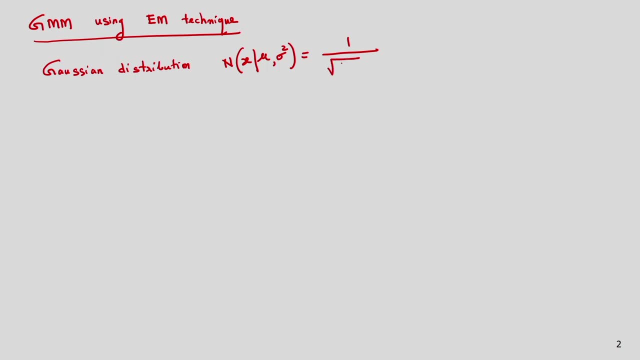 Any cond الص are usually no plus�âm, just one acting relation or ones picking the family長. Yes. So if youenever NOTHING, you are interested in knowledge about terms and parameters, then please stop and道ler. oh so it is 1 by twice pi. Sigma. square e to the power, minus X, minus mu, whole square 2 Sigma. 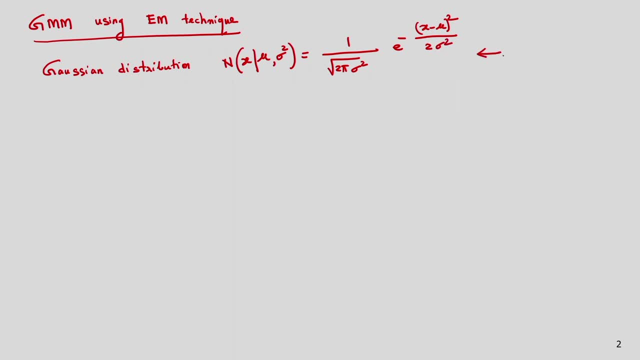 square. So this is the univariate Gaussian density. If I consider the multivariate normal distribution or the Gaussian distribution, that I can write like this: And X is a vector and I am considering the mean vector and the covariance matrix. this concept already i have explained in my previous classes. so 2 twice pi. 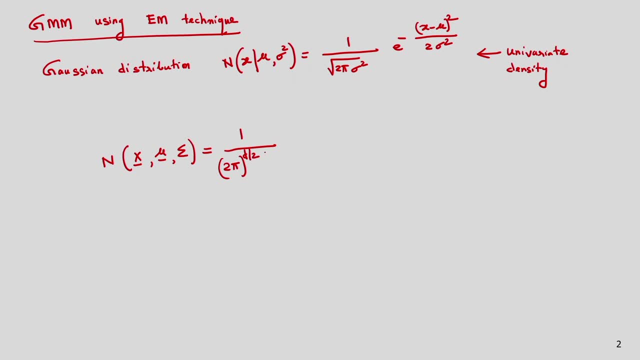 d by 2. so what is d? d is the dimension of the vector x, the exponential. so this is the expression for the multivariate density, the multivariate normal density. so we need to estimate the parameters of a distribution and for this we can consider the maximum likelihood estimation. 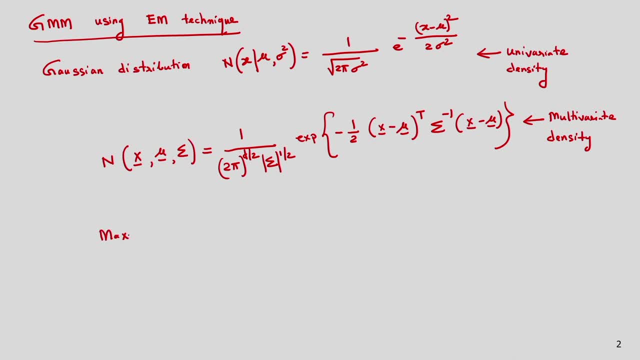 so this is a very, this is a very popular estimation technique. so we may consider the maximum likelihood estimation technique. so in this case i want to show you- suppose i have some data points- so this distribution i can represent by a gaussian function, that means by a gaussian distribution. 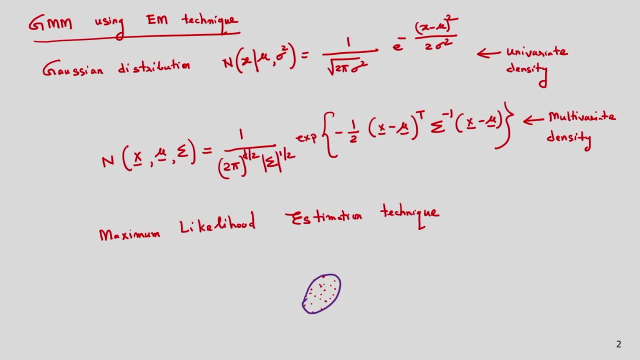 so if i consider this one, that is nothing but the gaussian distribution. if i consider the multidimensional case, i may get this type of ellipse: and this is the centroid. that means it is the mean of this gaussian. So that means this data distribution is represented by a Gaussian distribution, or 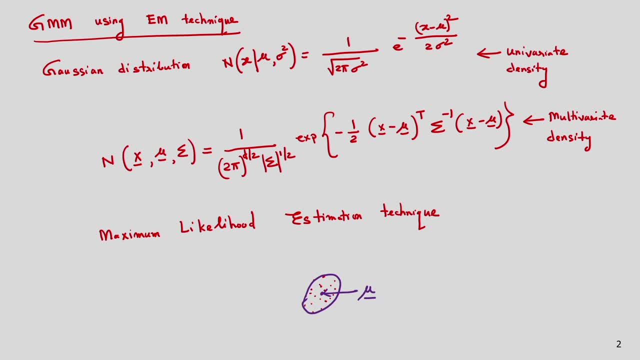 Gaussian function. So now, how to determine the values of the parameters. So already I told you we have to apply the ML technique, the maximum likelihood estimation technique. So move to the next slide. So what we need to consider: the log of Gaussian distribution. we have to consider in case 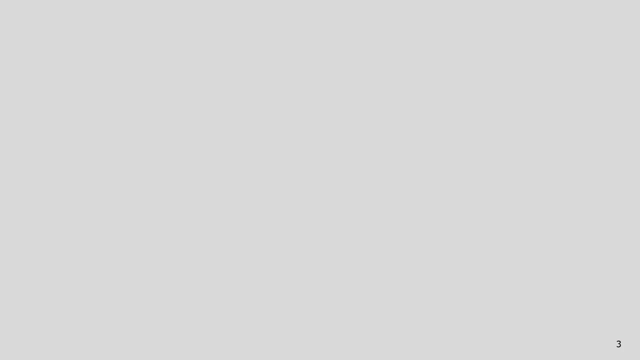 of the maximum likelihood estimation and take the derivative and equate it to 0.. So what I need to consider log of Gaussian distribution. first I have to take this one. after this, take the derivative. So after this I will be getting the values of the parameters. 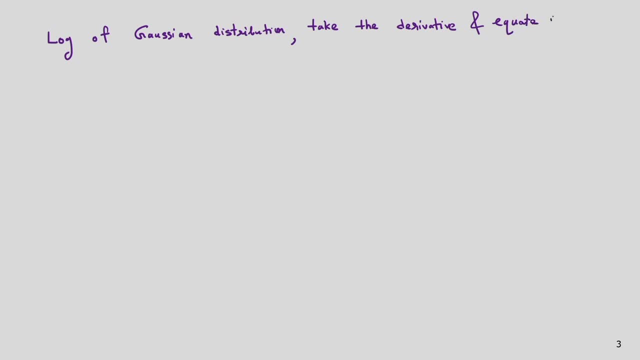 So mathematically I can write like this: I am taking the log of this density function X, mu. Okay, Okay. So sigma minus d by 2, ln, twice pi. this expression already I have explained in my discussion of Bayesian decision theory. 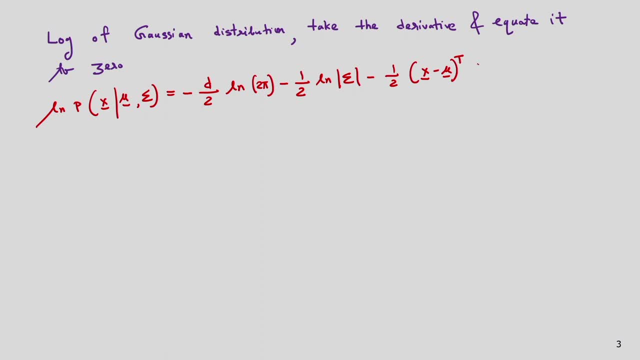 Okay, So we are taking the log of the Gaussian distribution and after this I have to take the derivative with respect to the parameter mu and equating it to 0.. And for the another parameter, that is the covariance matrix, Again I am taking the derivative. 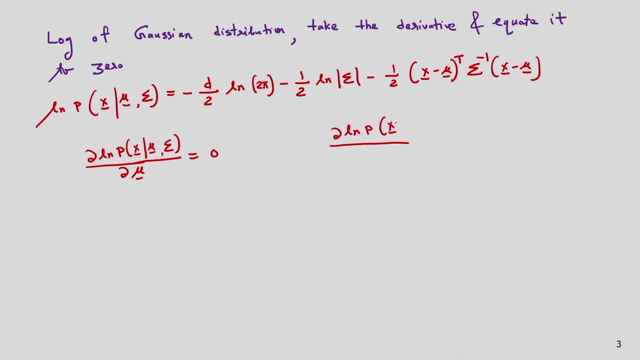 Okay, So I am taking the derivative with respect to the covariance matrix and equating it to 0.. So, corresponding to this one, I will be getting the mean, the estimated mean, by the maximum likelihood estimation technique. So that is 1 by n. summation n is equal to 1 to n. 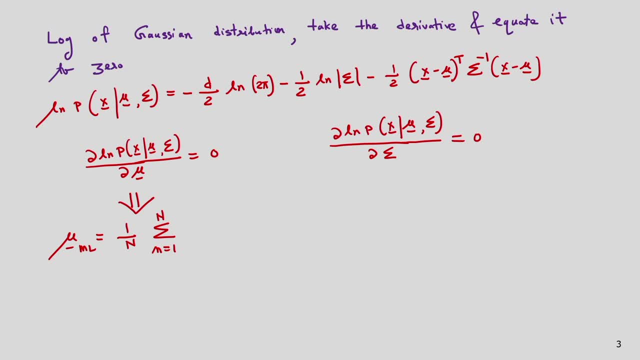 Okay, So we have n number of samples, or the data points X, n, And corresponding to this one, I have the estimate for the covariance matrix. So 1 by n, summation n is equal to 1 to n, X, n, mu, n. 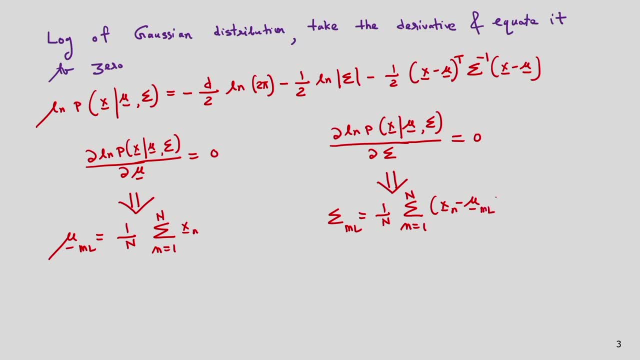 Okay. Okay, Now I have money which is 0. Okay, So I have the estimate for the covariance matrix. So the sum of n is greater than 1 by n. the pushup in 2000 is entonces 2셀 A super. 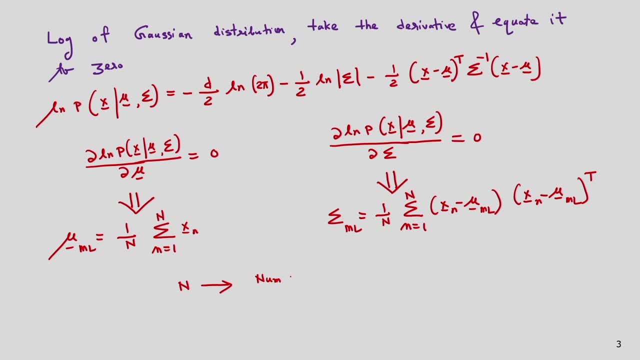 power, n by n is equal to 0. In other words, there is a confidence matrix. So I have the estimate for the covariance matrix. So here n is nothing but number of samples or data points, But number of samples is equal to n. in the case ofар egg, n is equal to n by n minus n. that is, n equals a power zero plus for n, which is 0.. Where n is essentially 1 by n is equal to n minus n squared in minus n. So you have m at parabola. n is equal to 0, it will mostly equal to n. 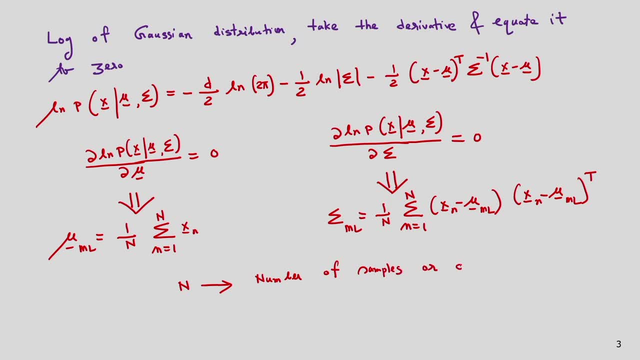 So it means that if I would fire shift at f, this is 0.. So this is about. this is about a Gaussian distribution and how to determine the or how to estimate the values of the parameters. Now let us discussed about the Gaussian mixture model. 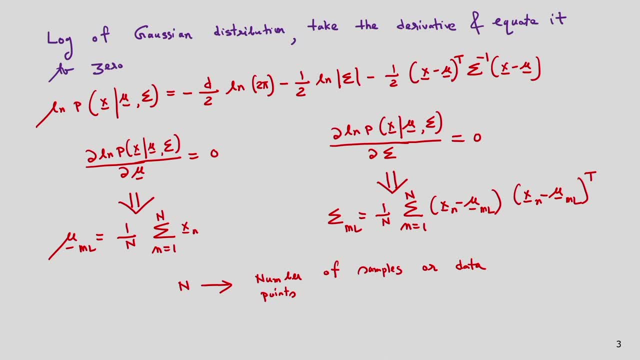 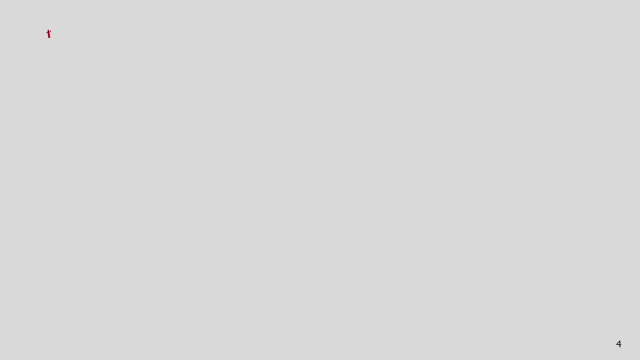 So why actually we need a mixture model? that concept I am going to explain in my next slide. So why actually we need a mixture model? Suppose I have some data points. these are the data sample points. So suppose I have some data points. 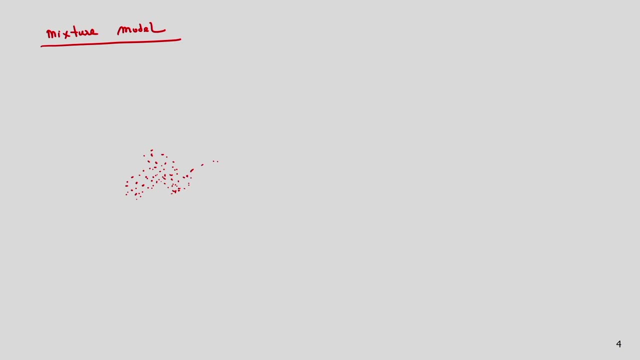 So we are considering this data set. So this data distribution it is not possible to represent by a single Gaussian. That means I cannot consider a single Gaussian distribution to represent this data distribution, So we have to consider multiple Gaussians. So in this case we may consider three Gaussians to represent the data distribution. 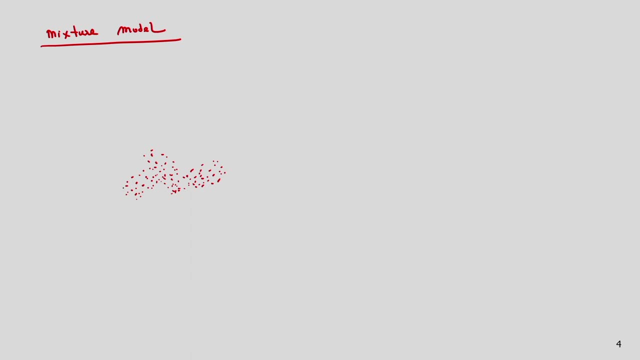 So maybe we can consider these, all these points we can consider. this will be one cluster and this cluster can be represented by one Gaussian. similarly, I may consider all these data points, So these data points or this data distribution can be represented by another Gaussian. 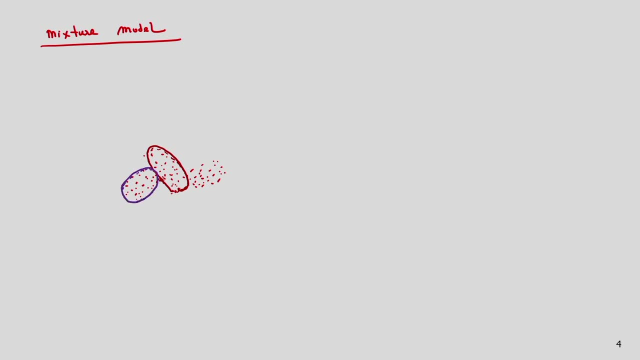 So this is one Gaussian and similarly the last one. if I consider all these data distribution, data points that can be also represented by another Gaussian, So three Gaussians I can consider. So that means So three clusters we can consider. 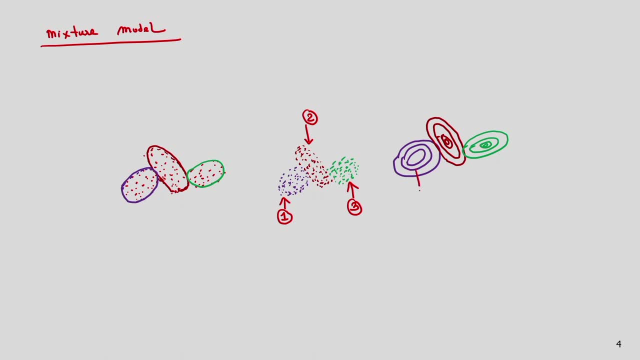 So these are actually the iso contours. So that means the distance from the mean is same for the iso contours, that is, the Mahalanobis. distance is same for all the iso contours. So we are getting three Gaussian and Gaussian one, Gaussian two, Gaussian three and that. 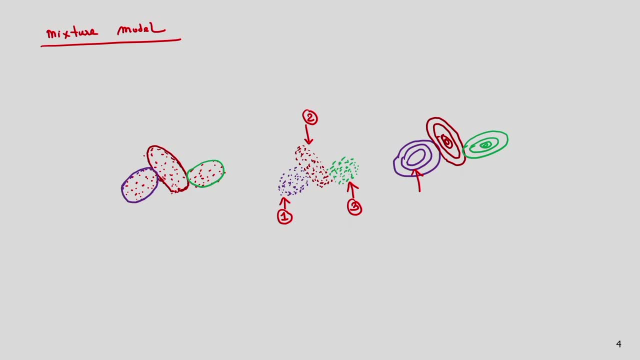 is the mixer model. that means the entire data distribution is represented, represented by a mixture model, the mixture of three gaussians. So in one dimension also we can show this one. So in one dimension, suppose, how to show this one? So first suppose 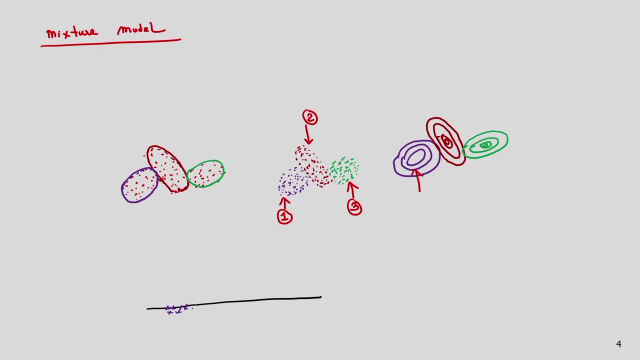 I have this data points. So, corresponding to this data point, I can consider one gaussian. Next, I have this data points corresponding to this distribution: I can consider another gaussian. Maybe I can consider another gaussian for this green color data points. So in 1D I can show like this, So you can see. that is the concept of the mixture model. 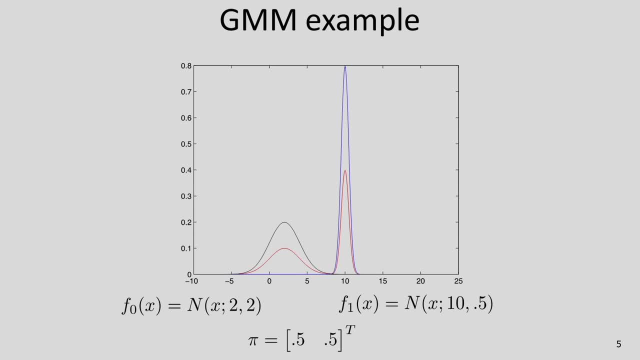 So in this case I am giving one example here. Here I am showing two gaussians. The first is represented by f naught, x, n, x, 2, 2.. So that is the first one. The first one is: it is shown by the black color. So the first one is: this is the first one. So this is: 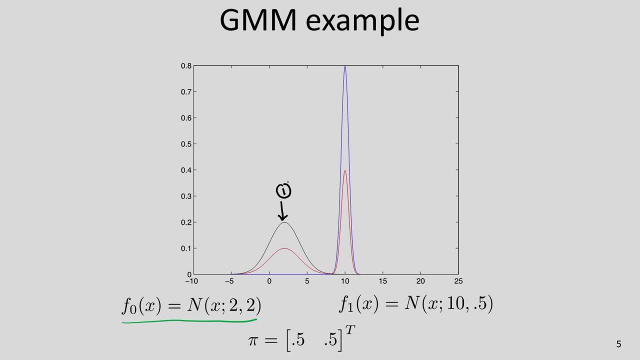 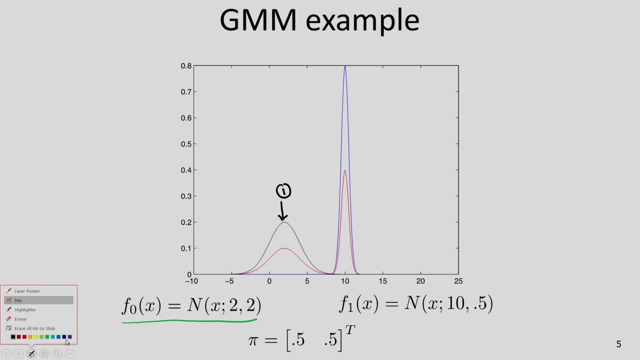 So for this I can show the gaussian is the blue color. So the second gaussian is number 2 gaussian and that is represented by the gaussian function f 1, x, and you can see the mean is 10.. So this is the first one for this gaussian and if you see the red one, that is actually 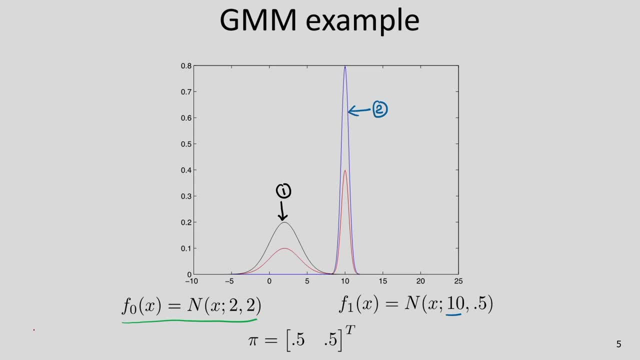 the combination of these two. The red one is the combination of these two. The red one is nothing, but it is 1 plus 2.. So we have to consider the linear superposition of gaussians. So this red one is nothing but the linear superposition of these two gaussians. So 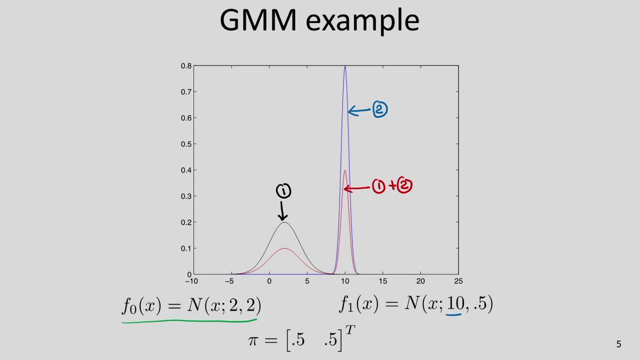 this is one example of a gaussian mixture model. So how to represent it mathematically? So move to the next slide. So suppose this gaussian mixture model, GMA m, how to represent mathematically this density? I can represent like this, because the mixture model is nothing but the linear superposition. 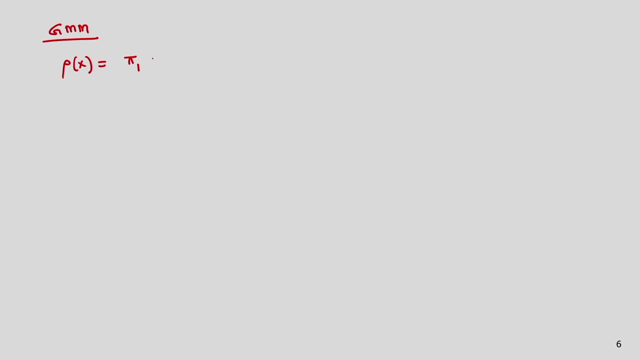 of gaussians, So pi 1 f 1 x plus pi 2 f 1 x, and by our getting here, by our gettingter, this is the linear superposition of gaussians. So pi 1 f 1 x plus pi 2 f 1 x plus pi 2 f 1 x. and here suppose the gefλέ. зачем this gaussian? 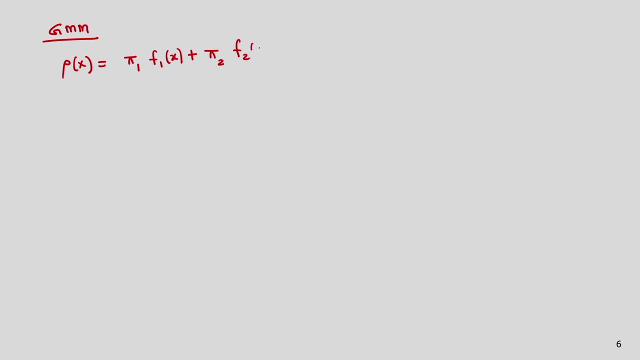 line an pale VIC 2 x plus pi, k, f, k, x. So here k means we are considering k number of Gaussians. So what is mixture model? The mixture model is the weighted sum of the mixtures of the pdfs, where 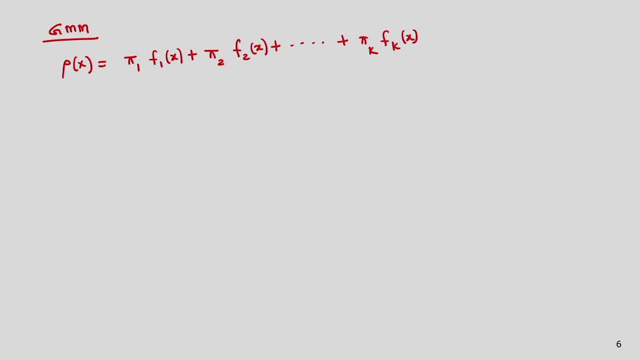 the weights are determined by a distribution. the distribution is pi. That means I can say the mixture model is nothing but the linear superposition of Gaussians. So here the mixing coefficient, the mixing coefficient that is the weight k is equal to 1 to capital K, pi. 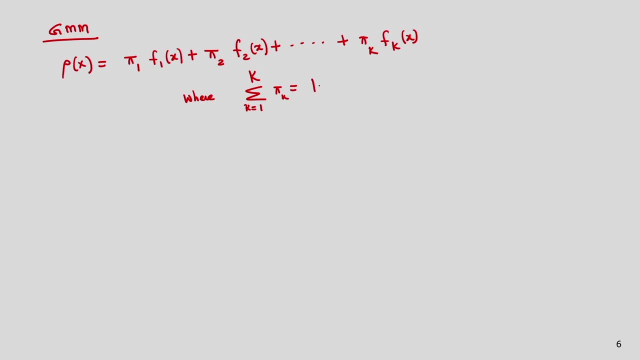 k, pi k is equal to 1.. So this can be written like this: summation: k is equal to 1 to k, pi, k, pi. pi is nothing but the mixing coefficient. pi is nothing but the mixing coefficient f, k, x. So this expression: 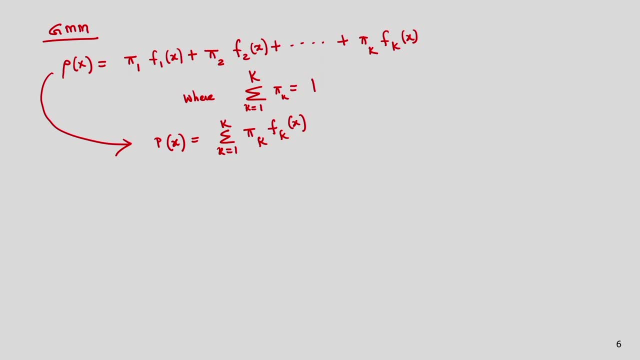 I can write in this form Here, this: f 1, x, that is nothing but the Gaussian density, that is the normal density. This density, I can write like this: pi 1, normal density. So it is x, mu 1, sigma 1.. I am not giving. 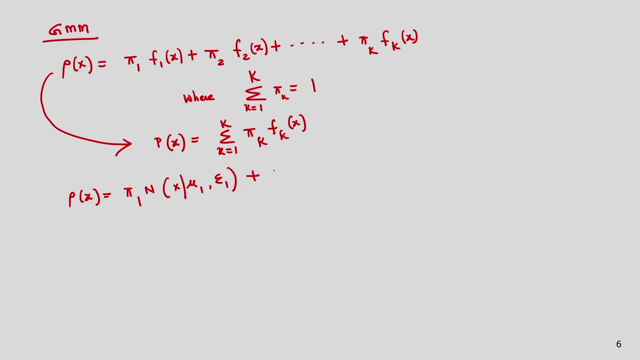 the vector sign here, mu 1, is nothing but a vector, but I am not giving the vector sign. So like this: I can consider number of Gaussians. So k number of capital, k number of Gaussians I can consider. 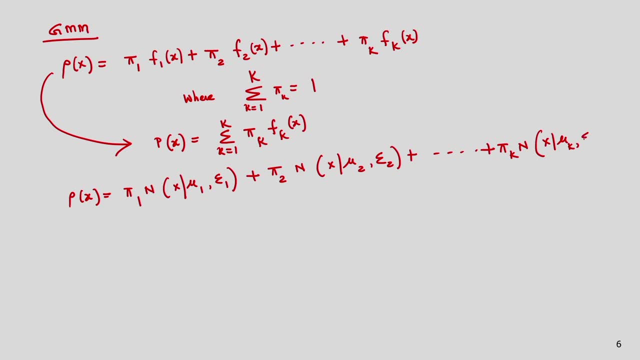 K number of Gaussians, So k number of Gaussians. I can consider k number of gaussians we are considering, so actually this expression also i can write like this: so in this case, the mixing coefficient: the mixing coefficient is pi k. 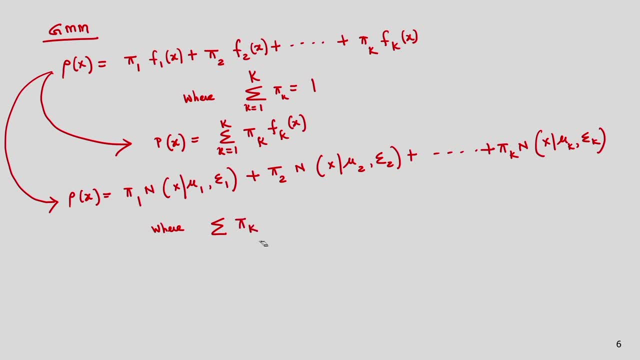 so mixing coefficient: pi k. so this small k, it is from 1 to capital k, so k number of gaussians we are considering. and finally, this expression i can write in this form: this is the mixer mixer of gaussian. so this is nothing but the mixer model. 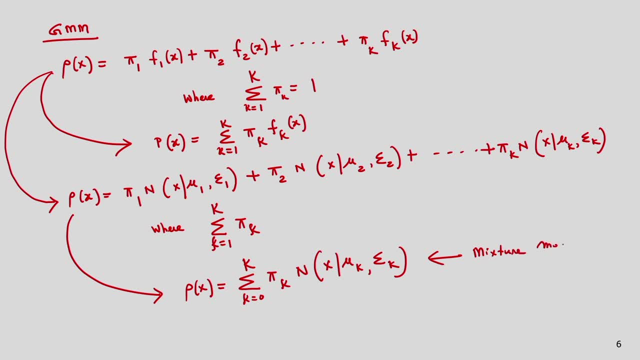 in this case we are considering k number of gaussians. so now we have to discuss the concept of the expectation maximization algorithm, because in case of the gmm, that is, the mixer model, i cannot apply maximum likelihood estimation technique to estimate the values of the parameters. 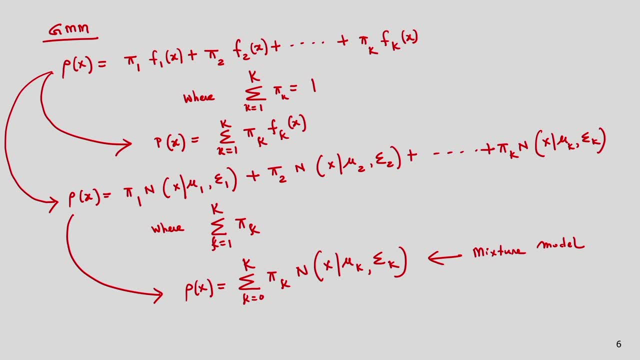 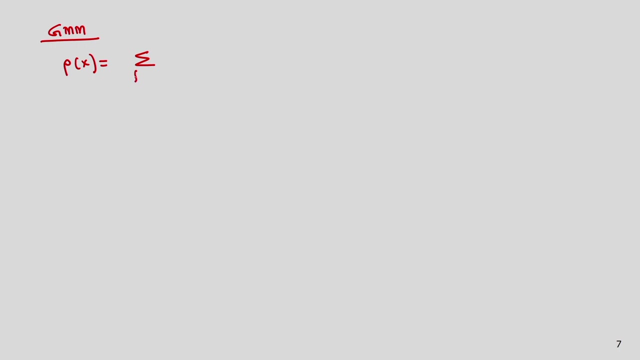 because i will not be getting the close form of the solution, so let us move to the next slide. so now we are discussing this gmm, the gaussian mixer model. so from the previous slide, how actually we are representing the density. we are representing like this summation: k is equal to 1 to capital k. k, number of gaussian. 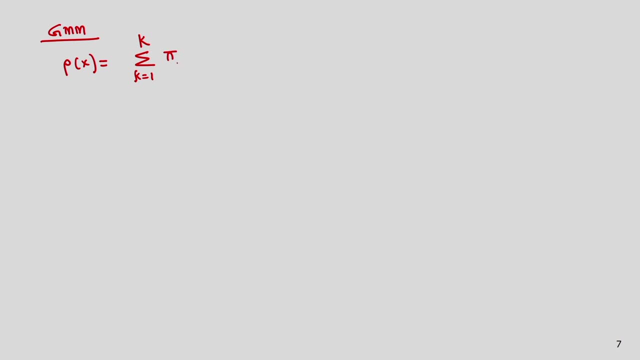 this is the weight, that is the mixing coefficient, and we are considering k, number of gaussians. i am not giving the vector sign. this x is a vector, mu is also a vector, so from the previous slide i can show like this: so in this expression this k is nothing, but it represents number of gaussians. 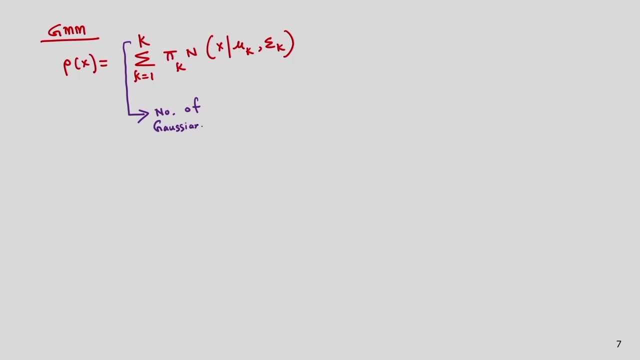 this pi k. it represents mixing coefficients or i can say weights- mixing coefficients or weights- and we have to consider some mixing coefficients or weights and we have to consider some conditions. that means we have to consider this normalization and also another condition is positivity. so these conditions I can write like this: the PI K, that is the 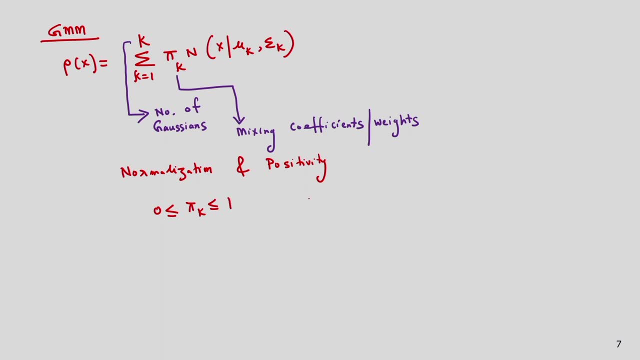 mixing coefficient lies between 0 and 1 and this K it is from 1 to K. PI K is equal to 1. so suppose if I want to determine the log likelihood, how to determine the log likelihood for of this? so this log likelihood also I can determine in maximum likelihood estimation. we. 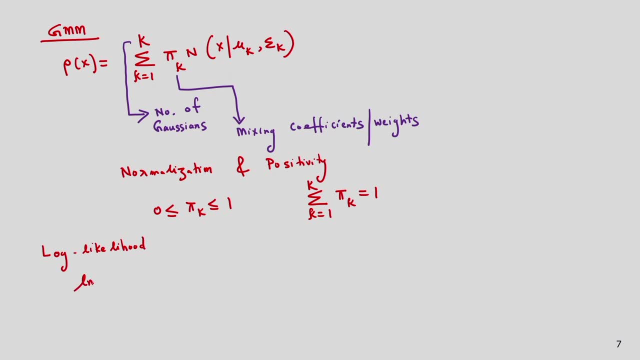 determine the log likelihood. in this case also I am determining the log likelihood. so you can see, here I have three parameters, one is mean, one is the covariance matrix, another one is the mixing coefficient. so three parameters we are considering mean. so you can see these three parameters I am considering mean: covariance matrix and 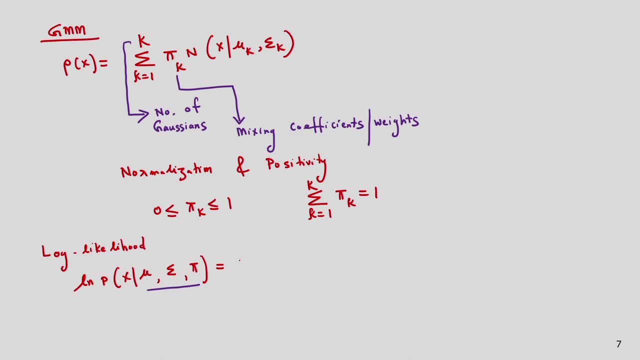 the mixing coefficient, summation n, is equal to 1 to n, ln. I can write like this: and this expression, it is equal to just putting the values of this density l, and k is equal to 1 to K, PI, k, n. just putting the value of this density l, n, this expression is equal to 0im divided by 0 line. in this case we have defined thisương correctly and the mixing coefficient lies between 0 and 1, and this expression is equal to 0. pi squared slows to 0. eighth, its the mean of L, nln 거예요. 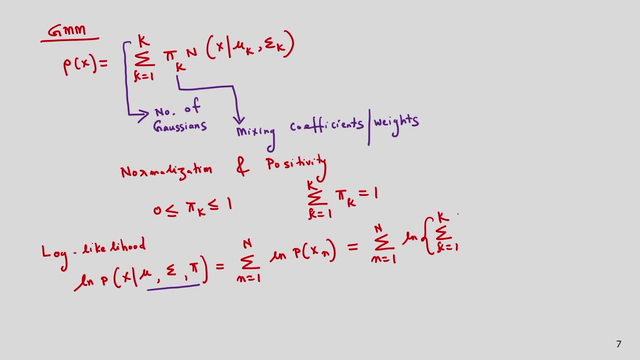 this expression is equal to just putting the values of this density ln, how you are to from error, K is equal to 1 to K. PI k n, just putting the value of this density- and anśli saw the見 point. and the mixing coefficient of k minus 1 to the N is equal to 0 pi squared. 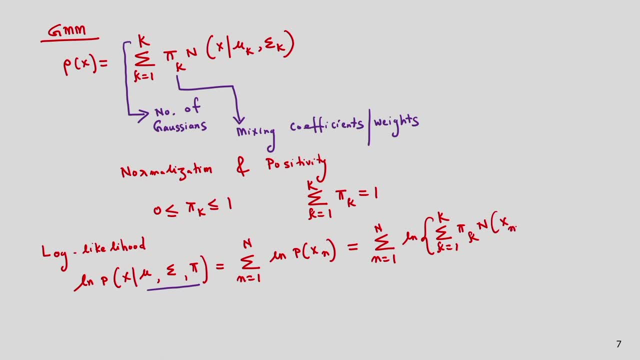 perfect. is that finished, Eiau? So this is the log likelihood. So this ML technique I cannot apply in this case because there is no close form solution. So this parameters can be calculated by considering EM algorithm. So move to the next slide. 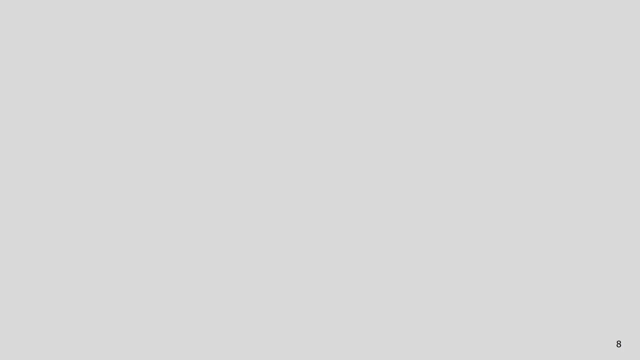 So we can think of the mixing coefficient as prior probabilities for the components. So this sentence I can better to write. So we can think of mixing coefficient as So for a given value of x, we can evaluate the corresponding posterior probabilities. 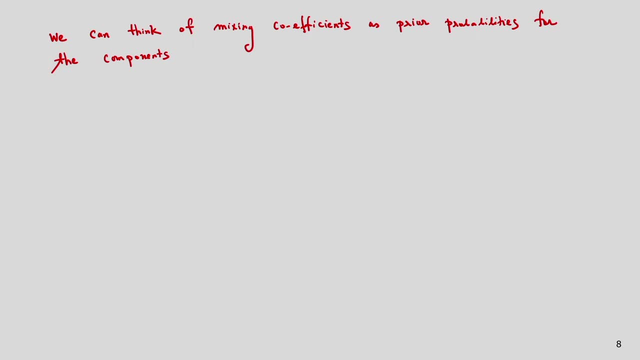 and which is called the responsibilities. So in the EM algorithm we are defining one term, that is the responsibilities. That means for a given value of x, we can evaluate the corresponding posterior probabilities and that is the responsibility. So from the Bayes, 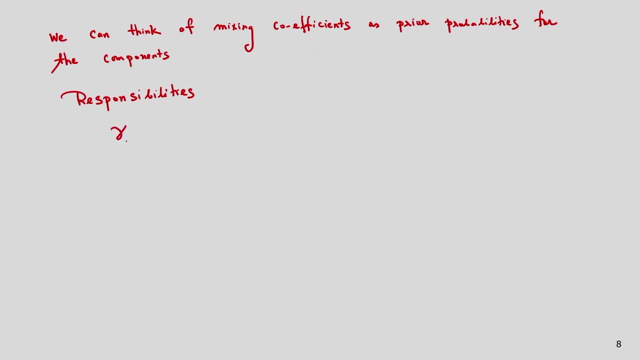 rule we are considering this gamma Kx. that is the responsibility and this is actually the latent variable we are considering. So by applying the Bayes rule, you can see, I can write like this: probability of K given x, that is the posterior probability. 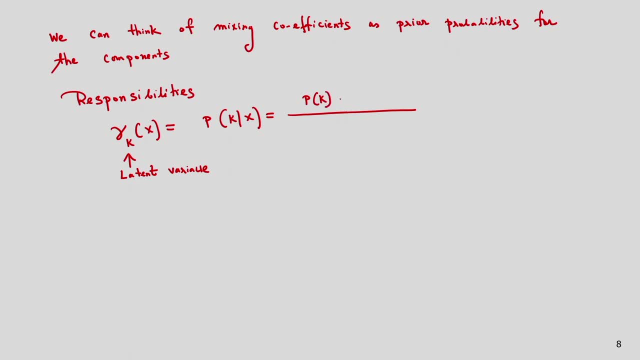 Probability of K, That is the class prior probability of K. is the class prior probability of x given K, that is the class conditional density. or this probability of x given K, that is the class conditional probability divided by probably of x, That is the unconditional prior So. 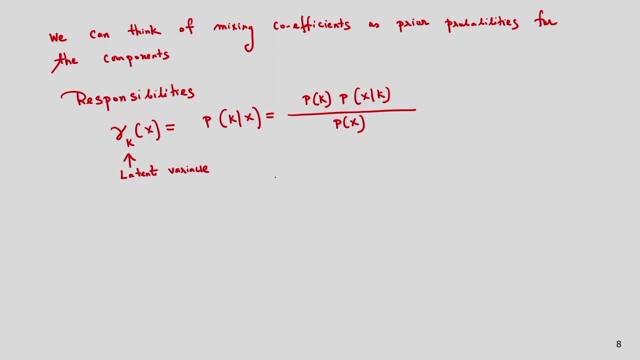 that's the unconditional prior. So this is by using the Bayes rule, So we can determine the posterior probability, probability of X given X. we can determine with the help of this, this formula. So now this class conditional density, I can write as a mixture of Gaussian: 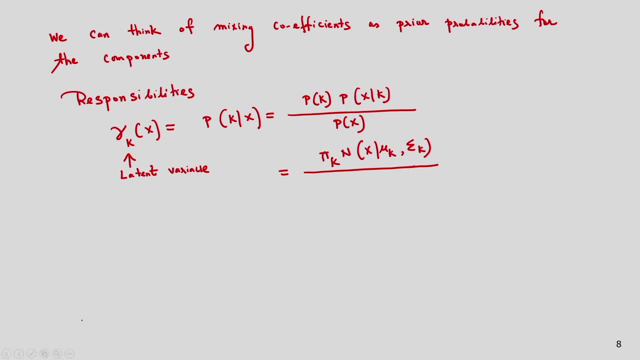 that means what we are considering, This class, conditional density, we are considering considering as a mixture of Gaussian and if I consider this denominator, we are considering the summation of all the Gaussians. So j is equal to 1 to k. k number of Gaussians: pi, j, n, X, mu, j. 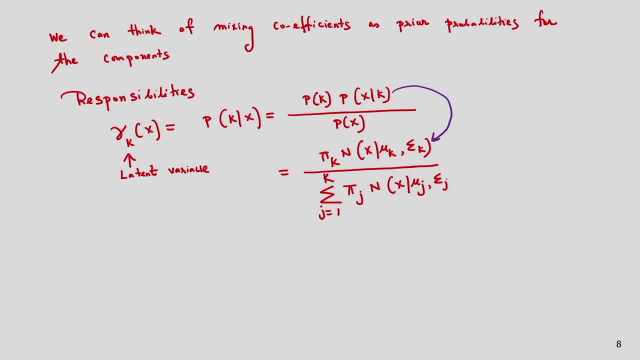 Okay, That is nothing but summation of all the Gaussians we are considering. So here pi k is nothing but n k divided by n. So here n k is nothing but number of points assigned. Okay, Okay, Okay. So in this way I can determine p, m to cluster k and capital N is nothing but total number. 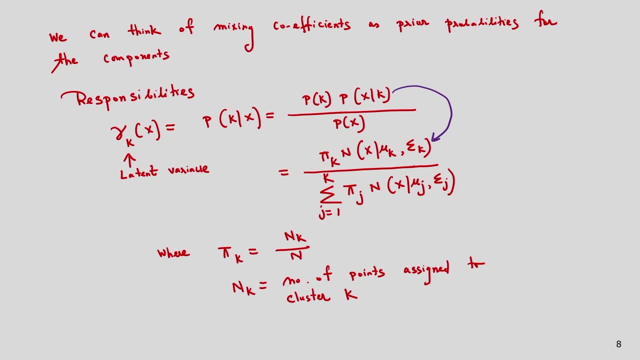 of sample points, all the data points. So, in case of the expectation maximization algorithm, this term is very important. the term is the responsibility. So we can determine the responsibility like this: This E m algorithm, that is actually the E m algorithm. 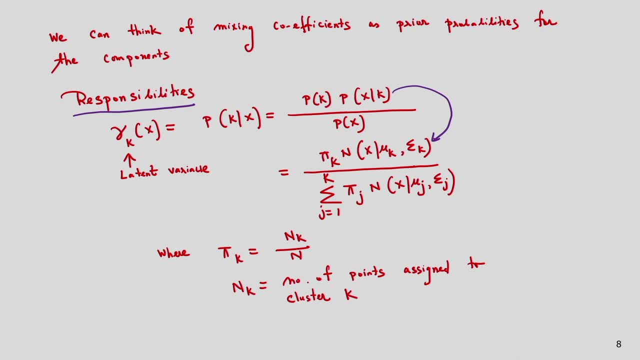 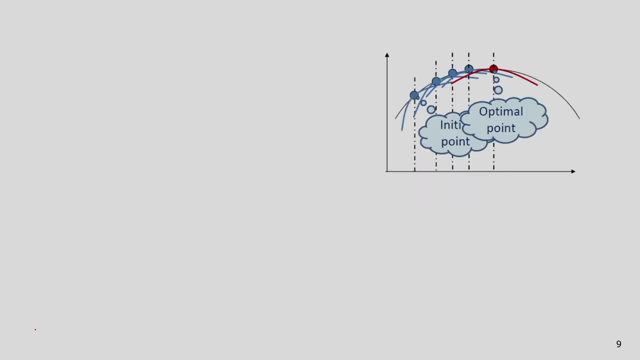 So if we talk about the reinforcement of E m, we can determine the form of the E m algorithm. that is actually the iterative optimization technique, which is operated locally. So let us move to this slide. So this expectation maximization algorithm, that is the iterative optimization technique. 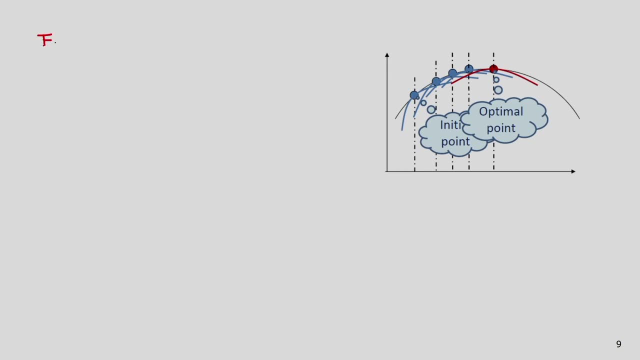 which is operated locally. So expectation maximization algorithm, this is the iterative optimization technique. So in the figure you can see: ah, this is the iterative technique we are, ah, we are applying. So you can see, ah, the we have initial point and after successive. 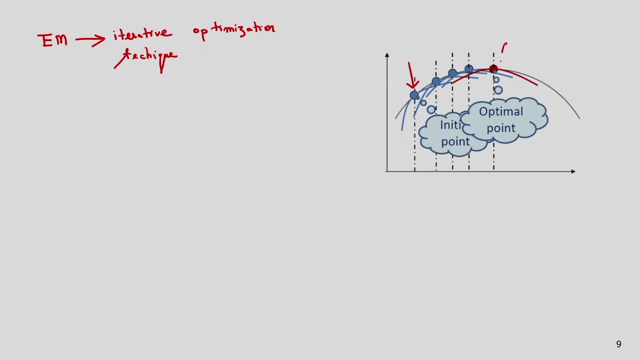 iterations we are getting the optimal point. So the final optimal point I am getting after successive iterations. So in this iterations there are two steps. one is the estimation step, another one is the maximization step. So in the EM algorithm I have two steps. one is the estimation step. 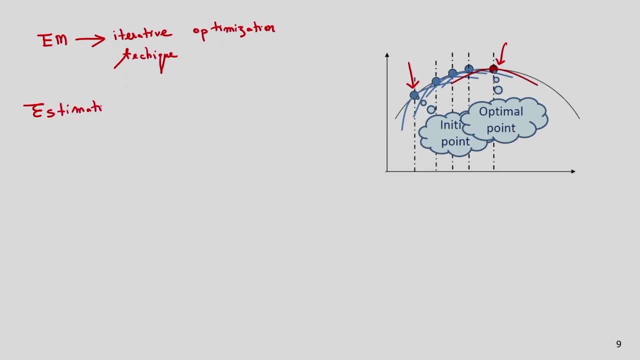 estimation step. So in the estimation step, what I need to do for given parameter values, U dance. So then I am going to compute the values like this. so, GU X, We can compute the expected values of the latent variable in previous Sãoü Raspberry. 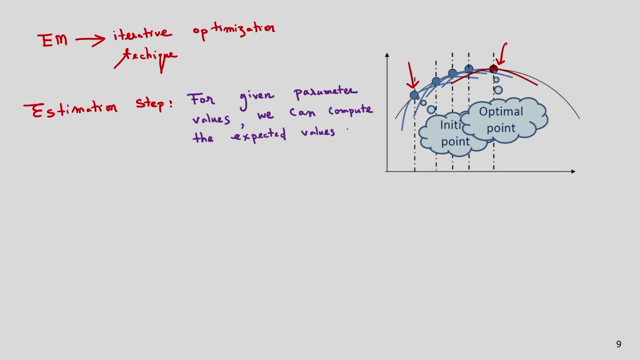 interval. That is nothing but the responsibilities. that is the expectation step. Next one is the maximization step. So in the maximization step, update the parameters of the model based on the latent variable calculated using ML method. 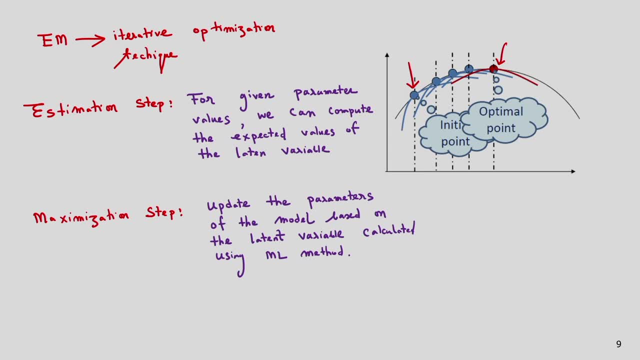 So this latent variable is nothing but the left hand responsibility. So update the parameters of the model. So what are the parameters of the model? The parameters of the model, Already I told you I have. the parameter is the mean, one is the covalent matrix. 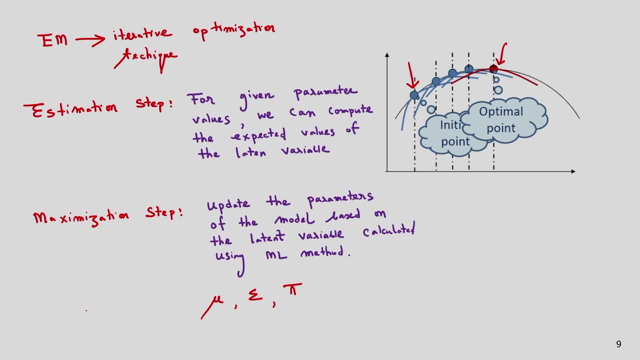 and another one is the mixing coefficients. So these are the parameters of the model, So these are the parameters. So the parameters of the model, sir, mean covariance matrix and a mixing coefficient. So first I have to determine the latent variable, first I have to determine the latent variable. 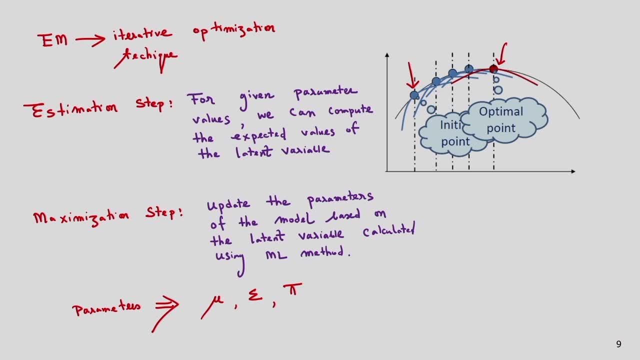 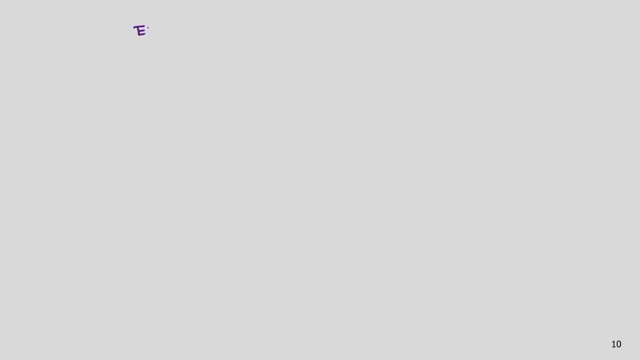 and after this, update the parameters of the model based on the latent variable calculated using ML method. so that is the concept of the expectation maximization algorithm. So now let us write the algorithm, that is the expectation maximization algorithm for the GMM. so EM algorithm for GMM: Gaussian mixture model. 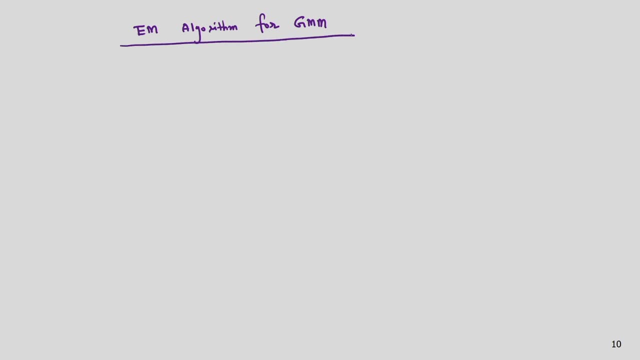 So I want to summarize this algorithm. The first step is number 1. Initialize the means mu j, covariance matrix, sigma j and the mixing coefficient pi j, So evaluate the initial value, values by likelihood. So one technique is: randomly we can select ah these values. 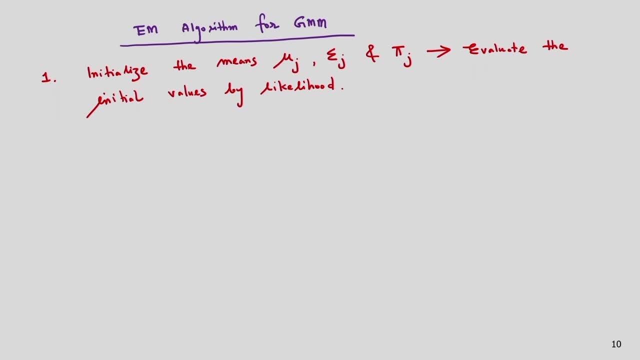 So initial initialize means initially we can select randomly the random values of these parameters And suppose, if I consider a data, So if I consider a data, So if I consider a data set or the data distribution, So I may consider the mean of this entire data distribution as the initial guess. or 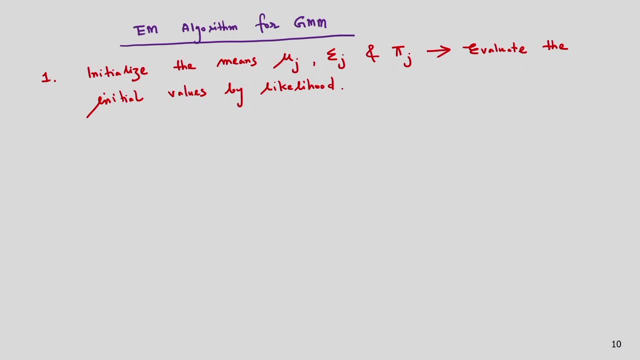 initial value. that also I can consider. but one technique is: randomly also, we can consider the values of these parameters initially. After considering this initialization, we have to go for the E step, that is the expectation step. What is E step? We have to evaluate responsibilities using the current parameter values. 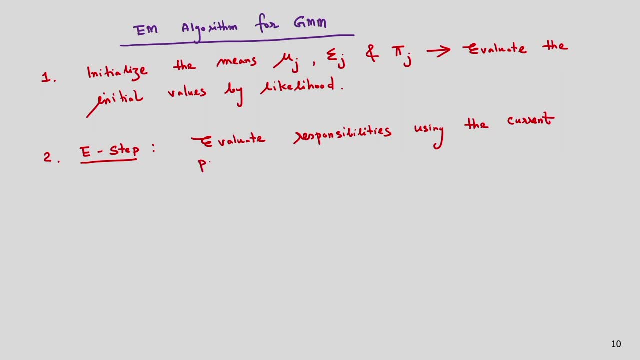 So this is the second step. After this, move to the next step, that is the third step, That is the M step, That is the maximization step. Re-estimate The parameters. 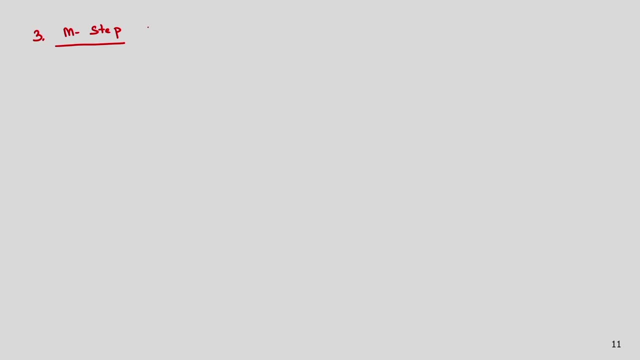 n is equal to 1 to n, the responsibility is gamma j, So this expression also it can be derived, but I have not shown the derivation. This is the expression for the mean, the expression. 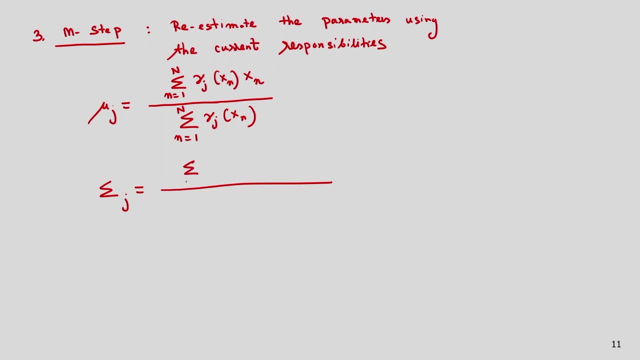 for the covariance matrix. Finally, I can determine the mixing coefficient, that is 1 by n. 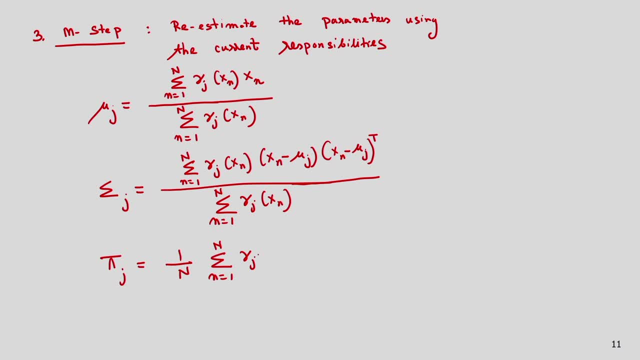 So these three parameters I can determine from the responsibilities. So all these three parameters I can determine from the responsibilities. And finally, ah, I have to converge. So the final step. I have to go for the convergence. So move to the final. 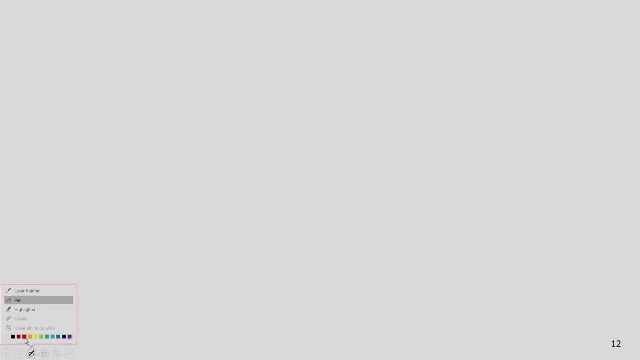 step. So for this, what we are considering, for the convergence, for testing the convergence of this algorithm, because this is the iterative algorithm. So evaluate log likelihood. So I have three parameters: mean covariance matrix and the mixing coefficient. So n is equal. 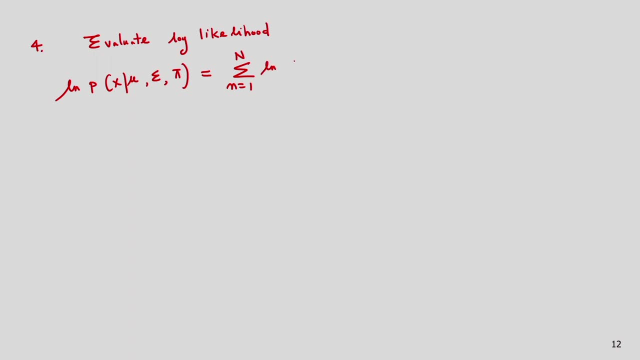 to 1 to n, n number of data points And we are considering capital, k number of gaussians. So correct, So we can determine the log likelihood. if there is there is no convergence, return to step 2.. So how to actually determine the convergence, Suppose I can consider the parameters. 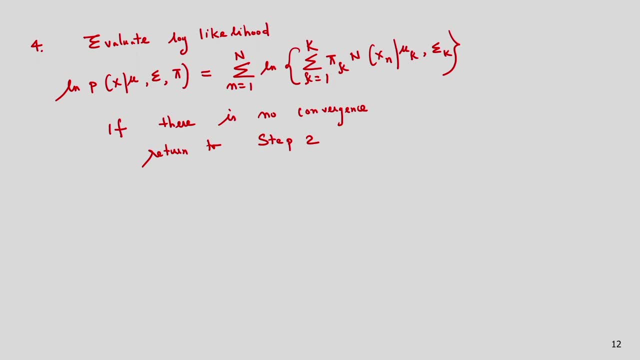 mean, covariance matrix and the mixing coefficient In two successive iterations. if there is not much changes of these values, of these parameters, that means I can stop the algorithm. I am repeating this So I can determine the mean, I can determine the covariance, I can determine the, I can 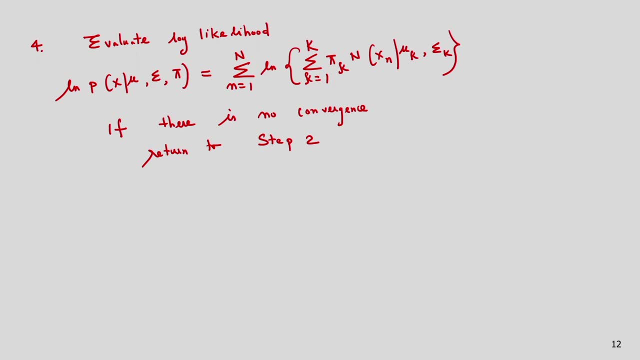 determine the mixing coefficients from the responsibilities And in two successive iterations. if there is no significant changes of the values of these parameters, then I can stop the algorithm. That is the condition for convergence. Another way also I can do, I can evaluate. 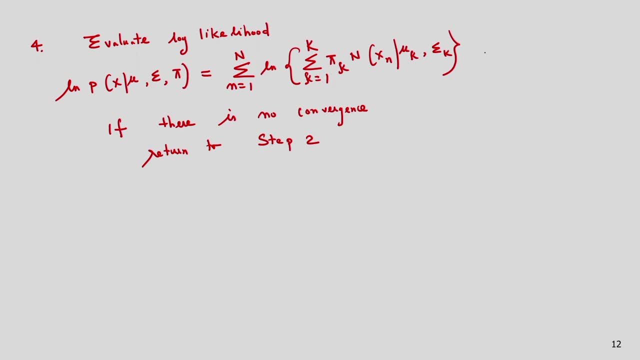 this log likelihood. Here you can see I am evaluating the log likelihood. So in two successive iterations If there is not much changes of this log likelihood value, then also I can stop the algorithm. That is the condition for the convergence. So based on the parameter values, I can take. 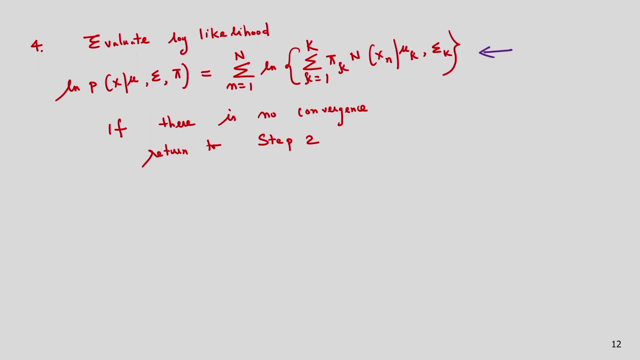 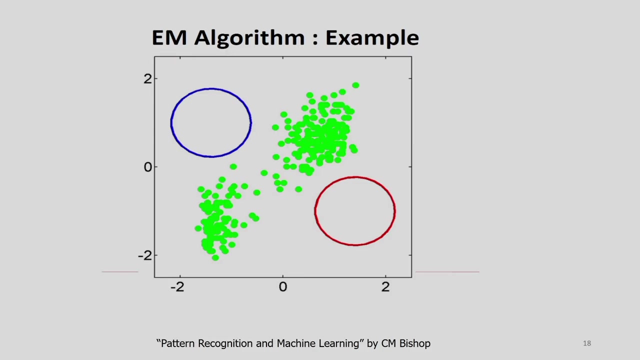 a decision And based on the log likelihood also, I can take a decision. So when to stop the algorithm? So because this is the iterative algorithm. So let us now consider one illustration of the expectation maximization algorithm. In this figure you can see I am showing a data distribution. So these are data points. 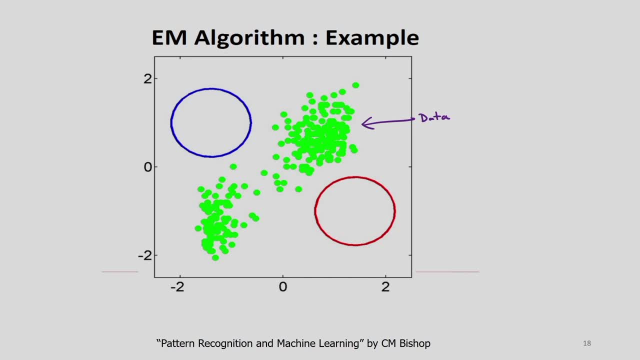 distribution of data, And with the help of single Gaussian it is not possible to approximate this data distribution. So that is why we have to consider number of Gaussian. In this case, I am considering 2 Gaussians: One is the red color, another one is the blue color. 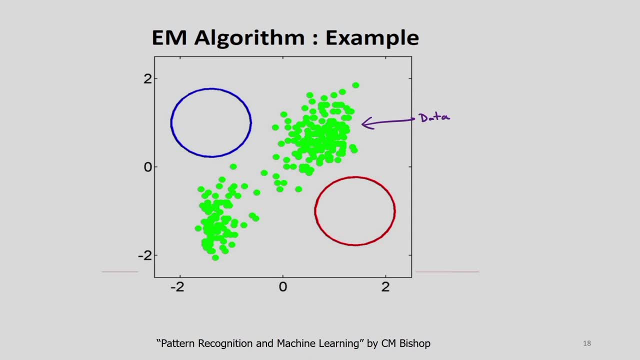 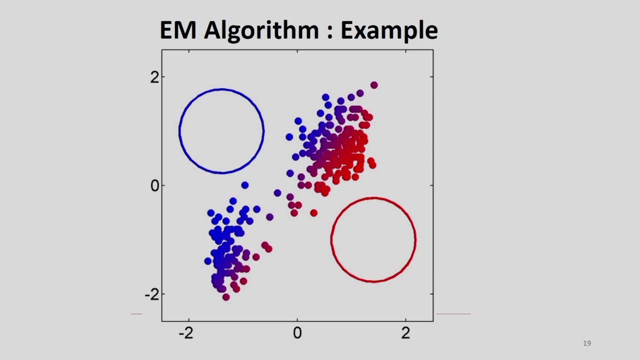 Gaussian clusters and suppose this is the initial position of these two gaussians. one is the blue, another one is the red and all the data points i have shown as a as green color data points. so move to the next slide. here you can see some of the points. data points are assigned to the blue cluster, that is, you can. 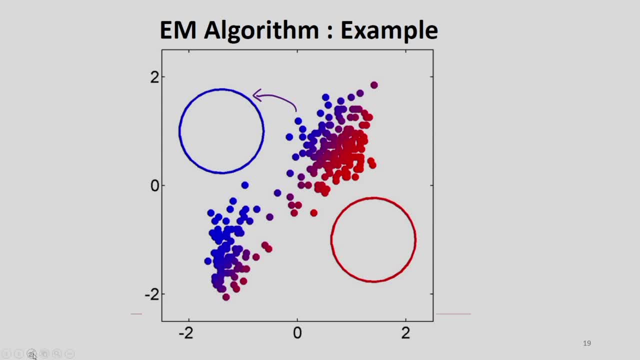 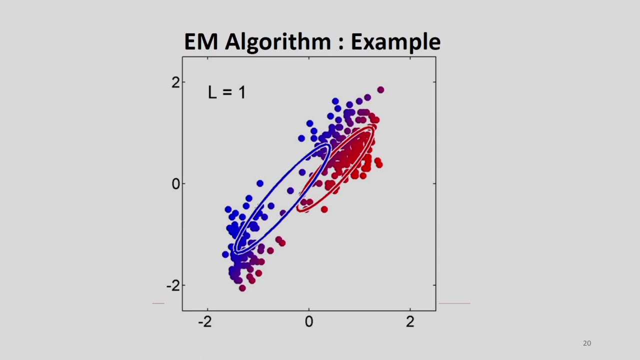 see, some of these data points are assigned to this, that is, the blue colored gaussian, and some of the data points are assigned to the, the red colored gaussian. so this is the initial assignment. so here you can see this is the. l is equal to 1 means this: 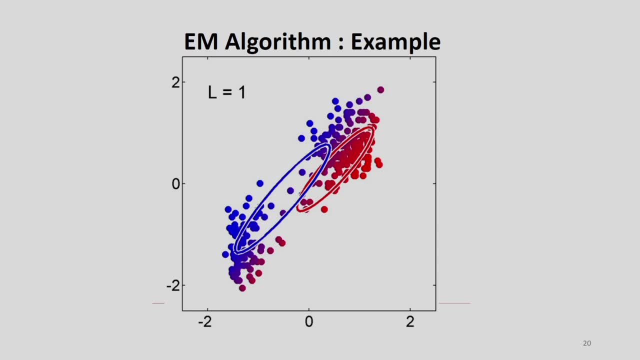 is the first iteration. after doing this, you can see i am getting these two new gaussians because i am assigning the some of the data points to the blue colored gaussian and some of the data points are assigned to the red colored gaussian and after this assignment main, I am having these two gaussians after the first iteration In the iteration number. 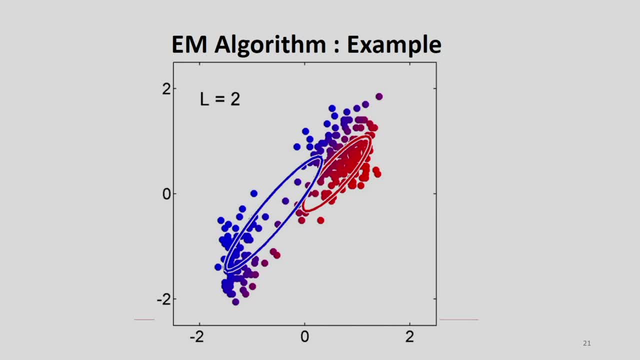 2, you can see the position of these two gaussians in the data set. So in the entire data distribution you can see the position of these two gaussians. after the second iterations. In the fifth iteration you can see the position of these two gaussians. One is the blue colored gaussian. 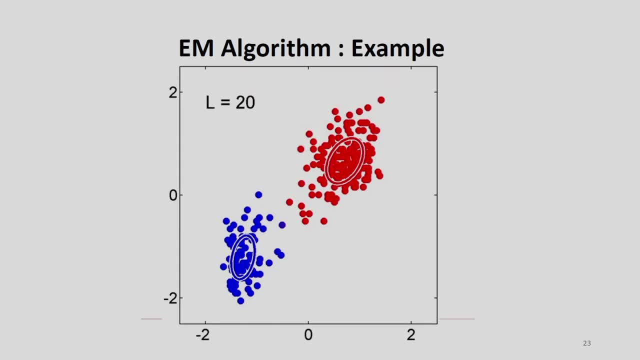 another one is the red colored gaussian And after 28 iterations you can see the final position of these two gaussians. So this blue colored gaussian can approximate these, all these data points, that is, all these data distribution, and the red colored gaussian can approximate all these data points. So that means, by considering these two gaussians, 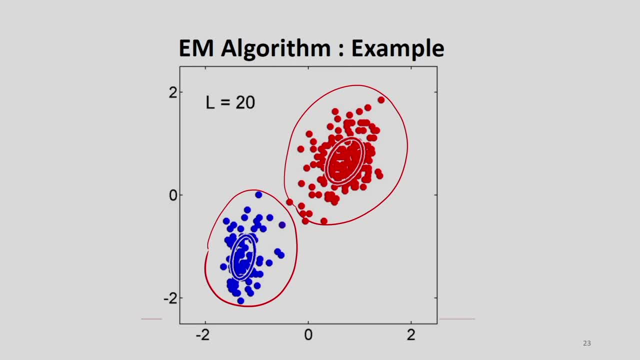 I can approximate this entire data distribution. So after this iteration I will be getting the convergence, Because not much changes in the values of the parameters. The parameters are already, I told you, the mean vector, covariance matrix and the mixing coefficients. So, based on 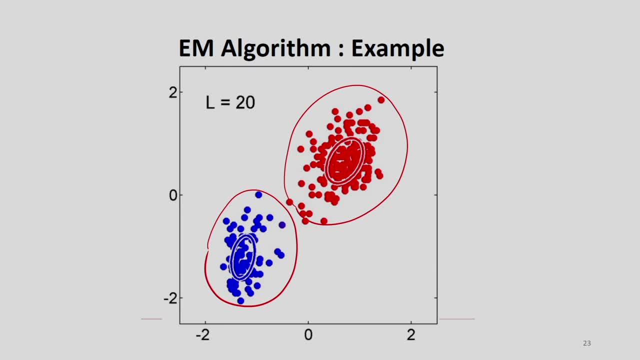 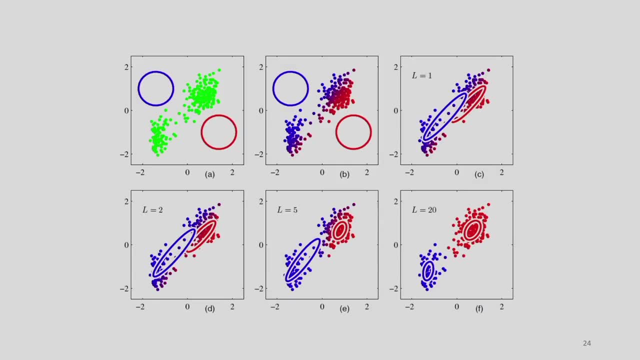 this I can determine the convergence condition, that is, I can stop the algorithm. So all the steps here I am showing together already I have explained. So initially I have shown two gaussians and after this, after the first iteration, you can see the position of these. 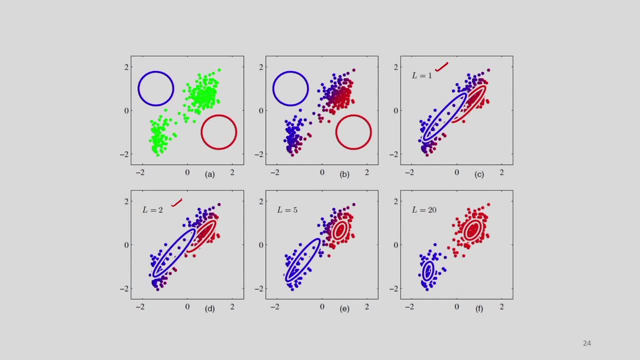 gaussians. After the second iterations, you can see the position of these gaussians like this: After the 20th iterations, you can see the position of these gaussians and after this I can stop the iteration, I can stop the algorithm. So this is the concept of the mixer model and 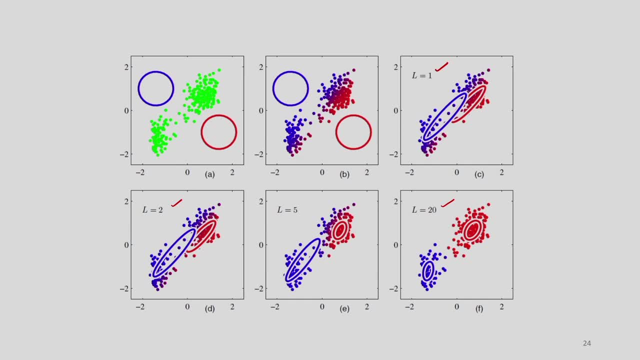 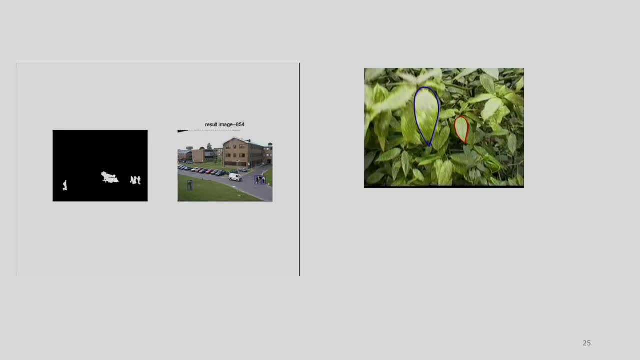 this is the concept of the expectation maximization algorithm. So one application of this algorithm I can show here: Computer vision. this computer vision application is: we can consider the segmentation problem, that is, the segmentation of foreground and the background. that is also called the background. 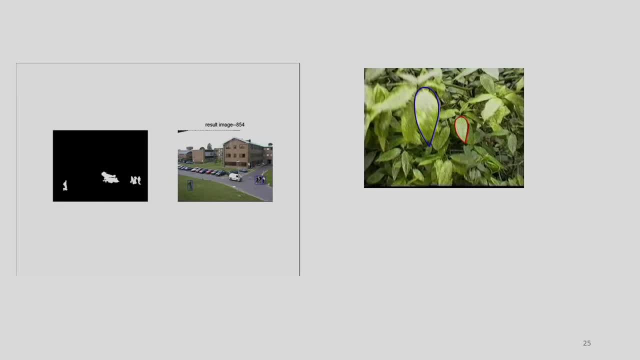 modeling and another one is the tracking. So the tracking of the object or the tracking- in this case I am considering the tracking of a leaf, And in this case you can see, suppose corresponding to this video, if I consider a, this particular pixel or these pixels. 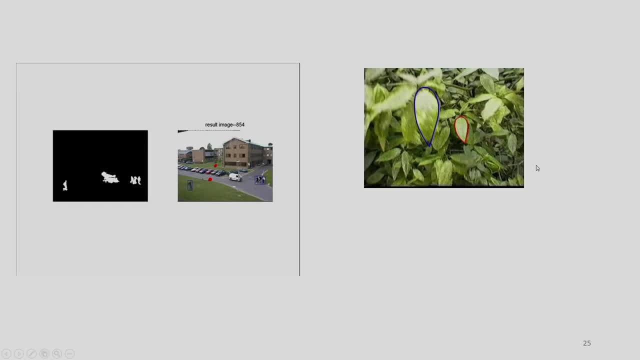 Because in a particular video I have number of frames and this pixel values. the distribution of this pixel values I can represent by a mixer of gaussian. Similarly, in the second case also, if I consider this point or any any one of the points, the pixel values, because 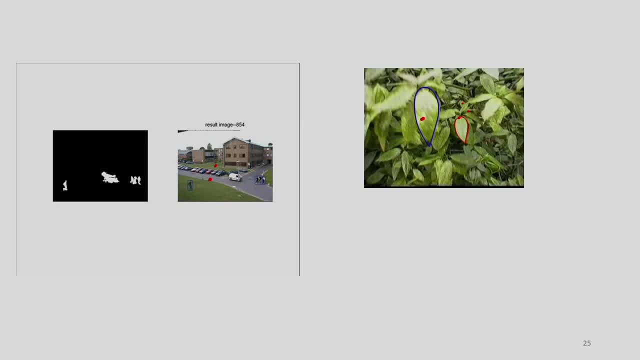 I have number of frames in the video, So the distribution of this pixel values I can represent by a mixer of gaussian And based on this I can develop a background. So this is the background modeling algorithm or may be the tracking algorithm I can consider. 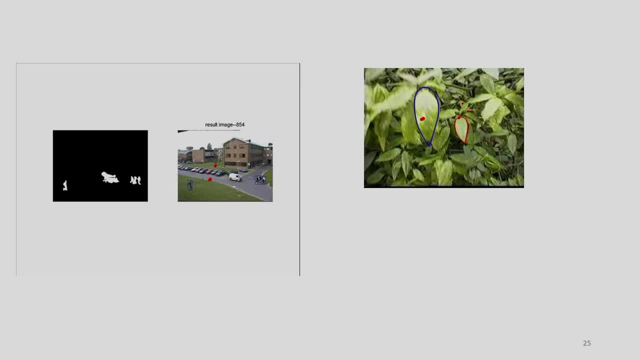 So this is one application of gaussian mixer model in case of computer vision application. So one is the background modeling, another one is the tracking. So here you can see I am playing this video and you can see just I am doing the segmentation. 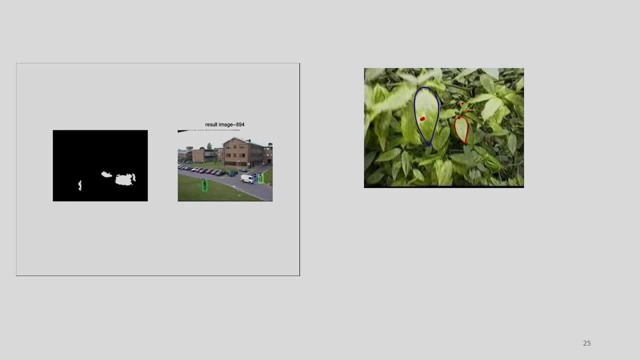 separation of the foreground and the background, And in this case for a particular pixel. So this is one application of gaussian mixer model. in case of computer vision application, We are considering the gaussian mixer model, the mixer of gaussians, because single gaussian cannot approximate the pixel distribution, the pixel value distributions. 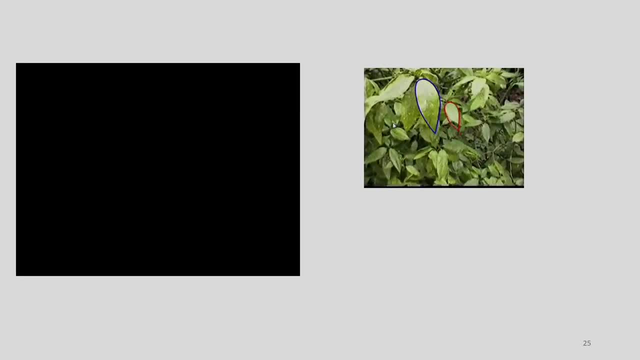 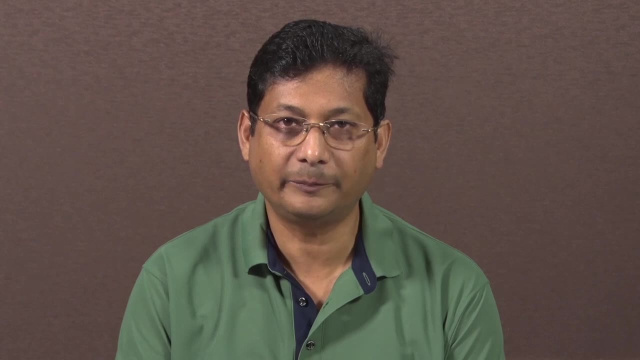 Similarly in the second case also, I can play this video. this is the tracking. In this case also, we have to consider the mixer model, the gaussian mixer model. So in this class I discussed the concept of the mixer model, What is the gaussian mixer model and why this gaussian mixer model is important for. 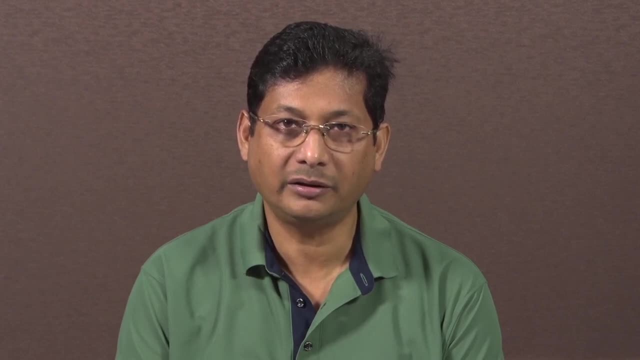 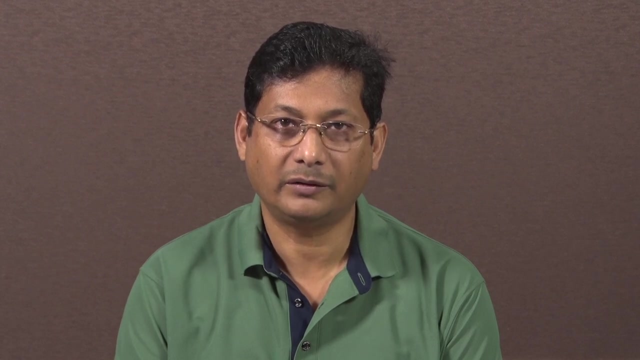 approximating a data set or a data distribution. that concept I have explained. After this I explain what is the problem of the maximum likelihood estimation to determine the values of the parameters in case of the mixer model, the gaussian mixer model, Because I will not get the close form of the solution. 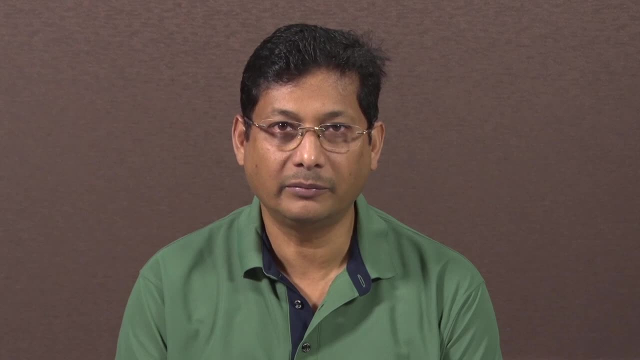 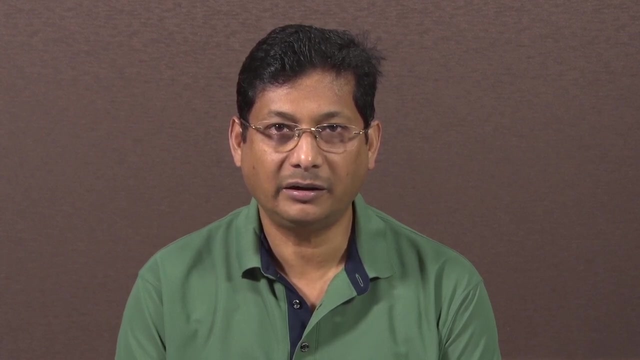 So that is why I have to consider The iterative algorithm, that is, the expectation maximization algorithm. In the expectation maximization algorithm, first I have to determine the responsibility and after this, with the help of this responsibility, I can determine the values of the parameters. 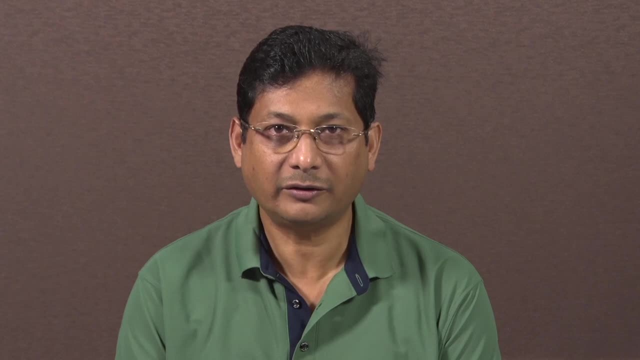 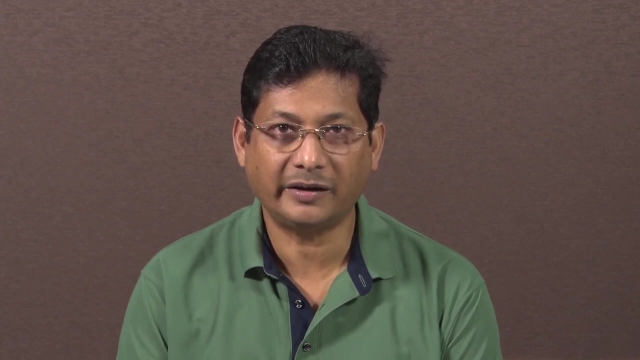 And this is the iterative algorithm and after this, based on some conditions, I can stop the algorithm. that is the convergence. I can consider the parameter values, the parameter means, the mean covariance matrix and the mixing coefficient and, based on this, I can stop the algorithm.